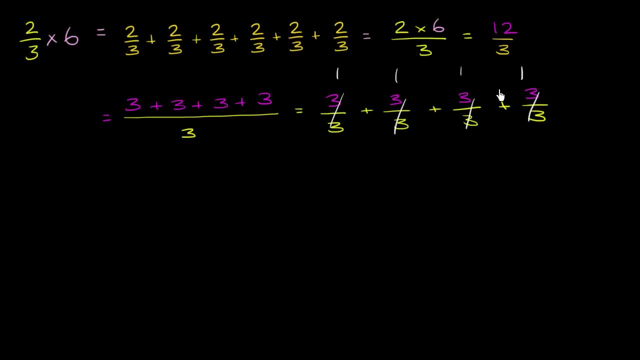 That's 1,, that's 1,, that's 1, and that's 1.. So this is going to be equal to 4.. So that's one way to conceptualize 2 thirds, 2 thirds times 6.. 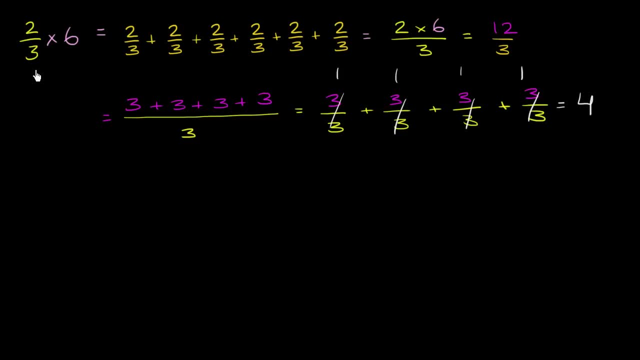 Another way to think of it is as 2 thirds of 6.. So let's think about that. Let me draw a number line here, And I'm going to draw the number line up to 6.. So what I care about is the section of the number line. 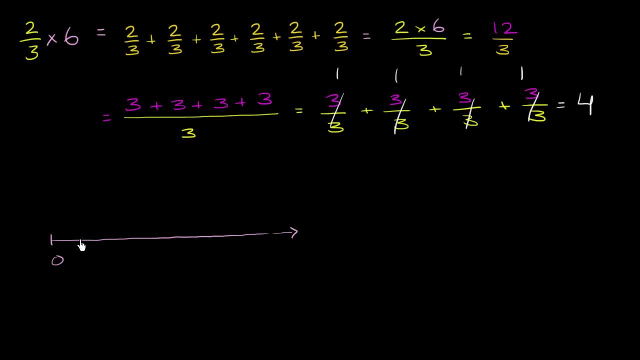 that goes to 6.. So that looks pretty good. So this is 1,, 2,, 3,, 4,, 5, and 6.. So if we want to take 2 thirds of 6, we're going to have 2 thirds of 6.. 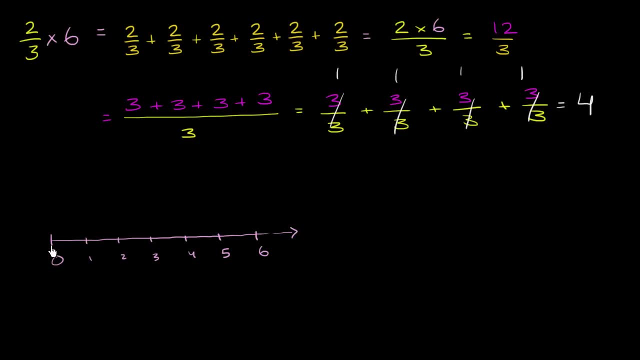 We can think of this whole section of the number line between 0 and 6 as the whole, And then we want to take 2 thirds of that. So how do we do that? Well, we divide it into thirds to 3 equal sections. 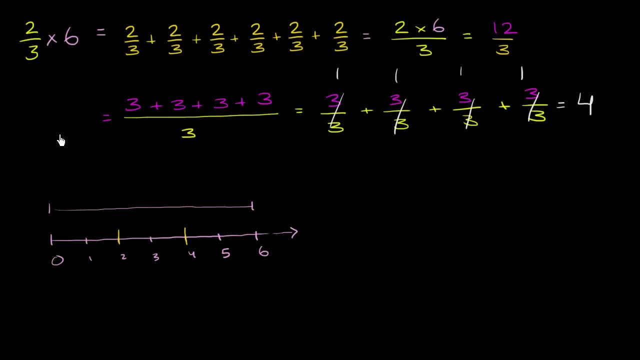 So that's 1 equal sections, 2 equal sections and 3 equal sections, And we want 2 of those thirds. So we want 1 third and 2 thirds. Now where does that get us? That gets us to 4.. 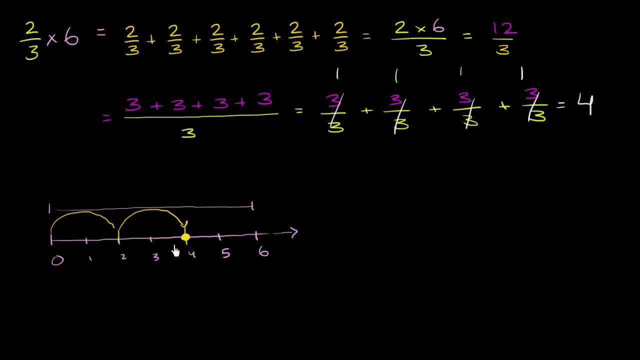 That gets us to 4.. So we get obviously to the same answer. It would be a tough situation if somehow we got two different answers, Either way: 2 thirds times 6, or 6 times 2 thirds. either way that is going to be equal to 4.. 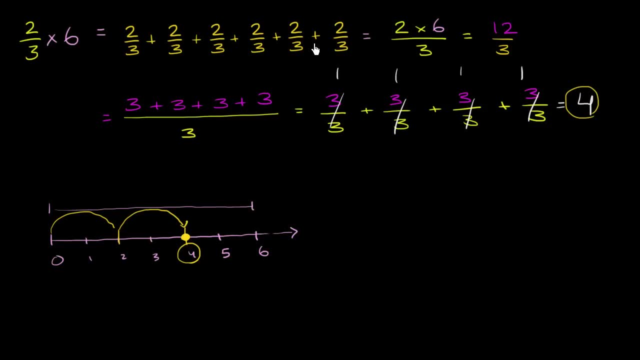 But there are two different ways of viewing this. This first way is literally viewing it as 2 thirds, 6 times, And this way is we're taking a fraction of the number 6.. We're going 2 thirds of the way to 6,, which would get us to 4.. 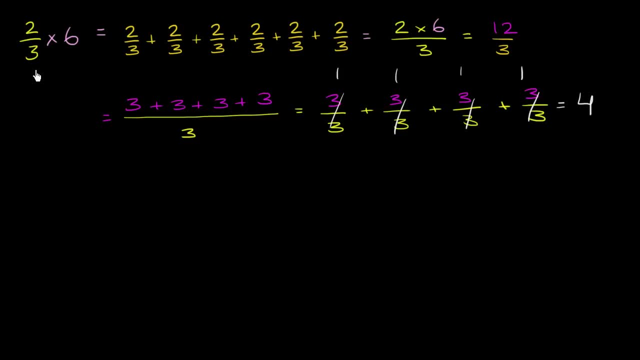 Another way to think of it is as 2 thirds of 6.. So let's think about that. Let me draw a number line here, And I'm going to draw the number line up to 6.. So what I care about is the section of the number line. 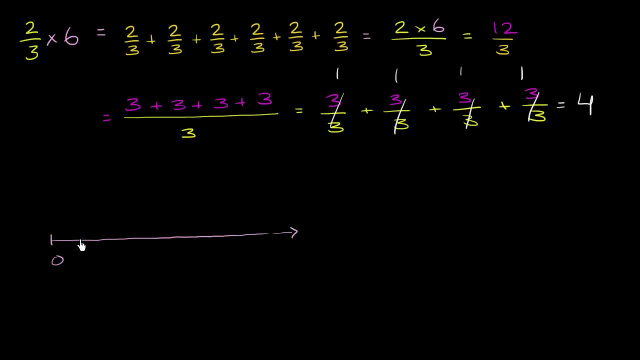 that goes to 6.. So that looks pretty good. So this is 1,, 2,, 3,, 4,, 5, and 6.. So if we want to take this, If we want to take 2 thirds of 6,, we 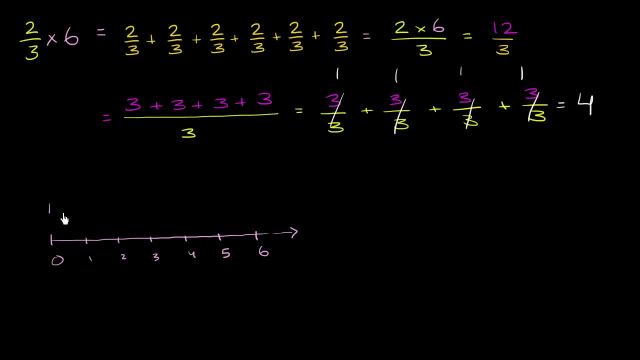 can think of this whole section of the number line between 0 and 6 as the whole, And then we want to take 2 thirds of that. So how do we do that? Well, we divide it into thirds to 3 equal sections. 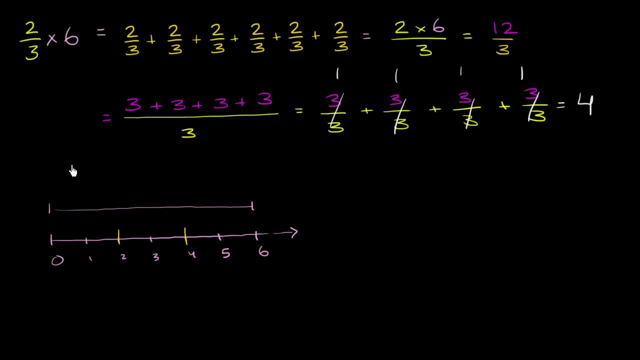 So that's 1 equal sections, 2 equal sections and 3 equal sections, And we want 2 of those thirds. So we want 1 third and 2 thirds. Now where does that get us? That gets us to 4.. 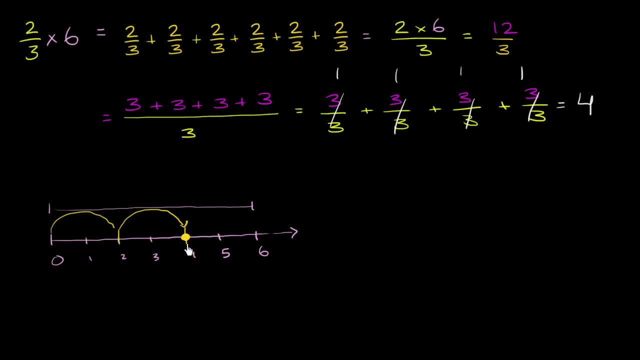 So we get obviously to the same answer. It would be a tough situation if somehow we got two different answers. Either way 2 thirds times 6, or 6 times 2 thirds. Either way that is going to be equal to 4.. 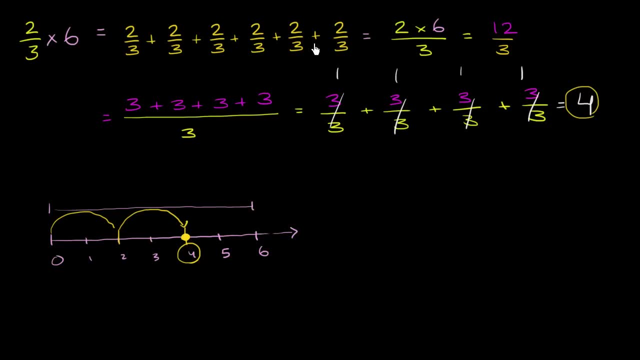 But there are two different ways of viewing this. This first way is literally viewing it as 2 thirds, 6 times, And this way is we're taking a fraction of the number 6.. We're going 2 thirds of the way to 6,, which would get us to 4.. 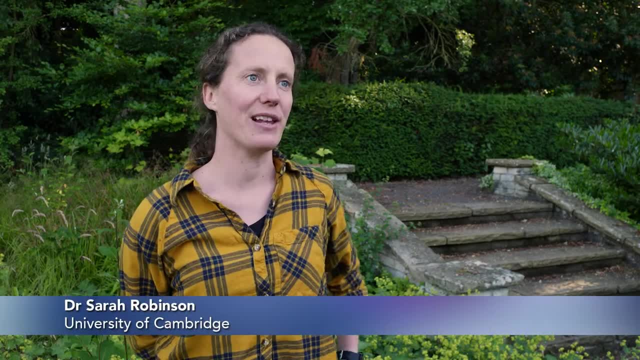 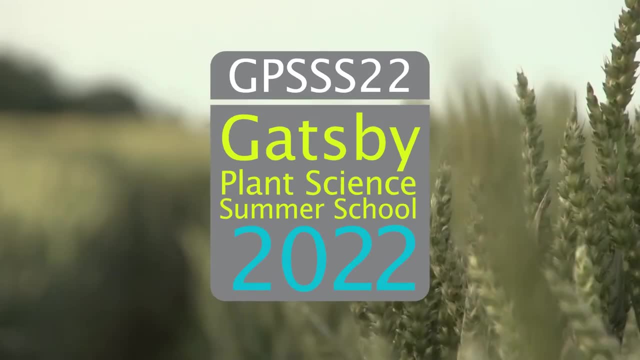 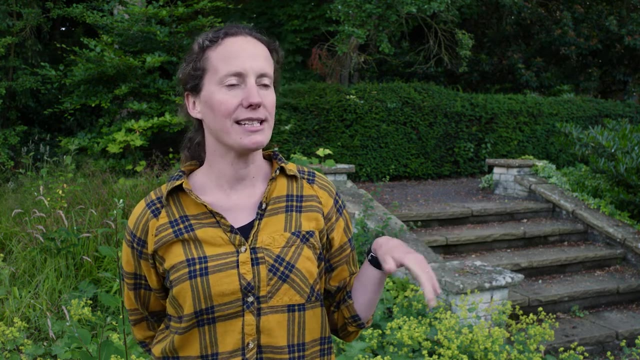 I'm Sarah Robinson. I work in the Sainsbury Laboratory. I work on plant development, mostly from a mechanical point of view, So my main research is how plants grow to create the shapes that they have. Particularly, we're looking at cell division versus cell expansion, which are the two things that control. 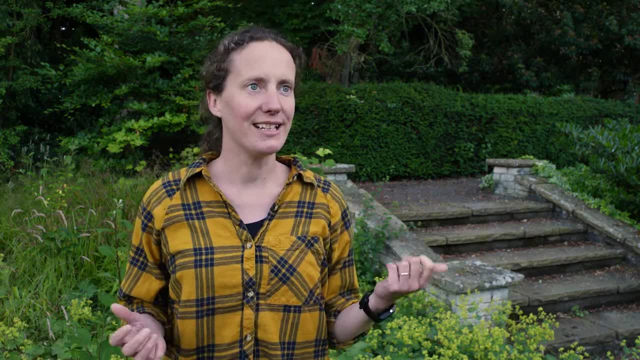 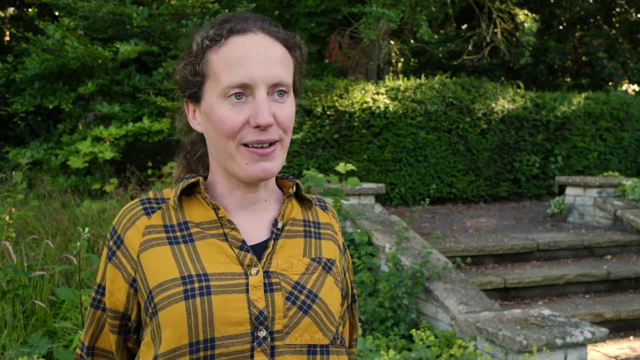 growth, And so we're looking at the trade-offs between those two processes and how they interact with each other. I do curiosity-driven research, so I like to understand how plants grow, how they develop, how they obtain the size and shape that they have, and the different processes.